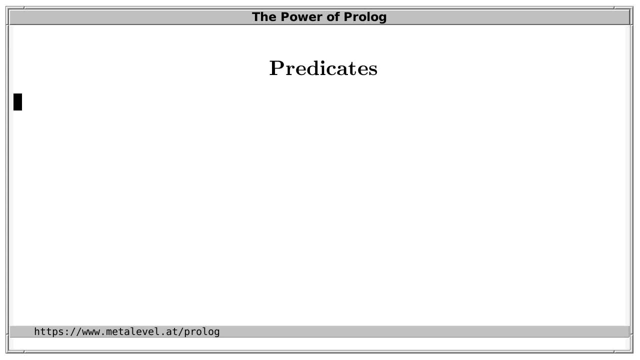 In Prolog you write programs by defining predicates. A predicate has a name and a number of arguments. The number of arguments is called the arity of the predicate. We write p slash n to denote a predicate with name p and n arguments. p slash n is called a predicate indicator. 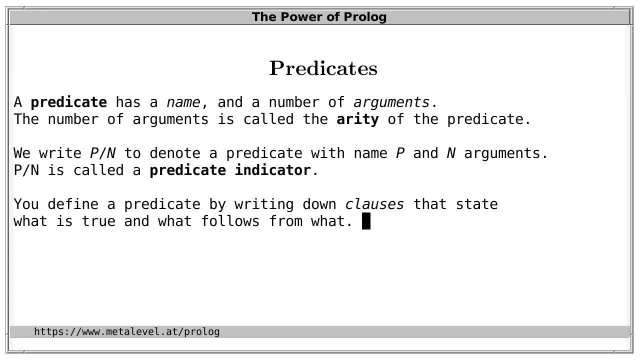 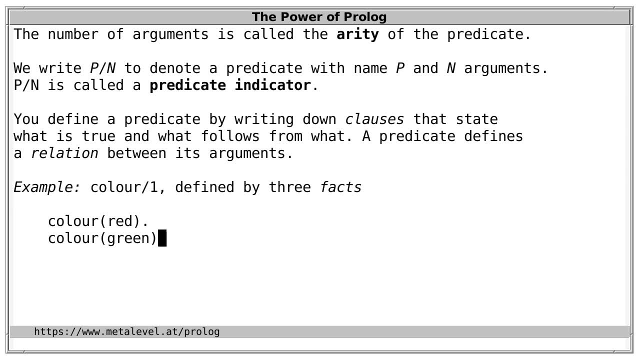 You define a predicate by writing down clauses that state what is true and what follows from what A predicate defines a relation between its arguments. For instance, here is a definition of the predicate color defined by three facts. These facts simply state that red is a color. 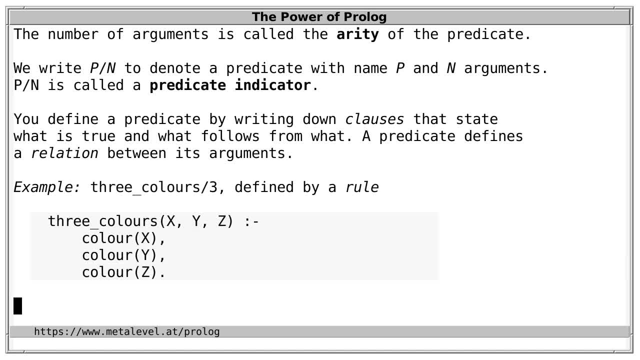 green is a color and blue is a color. And here is the definition of another predicate: three colors with three arguments, defined by a rule. This states that three colors of x, y and z holds. if x is a color, y is a color and z is a color. Now, when you start your Prolog system, 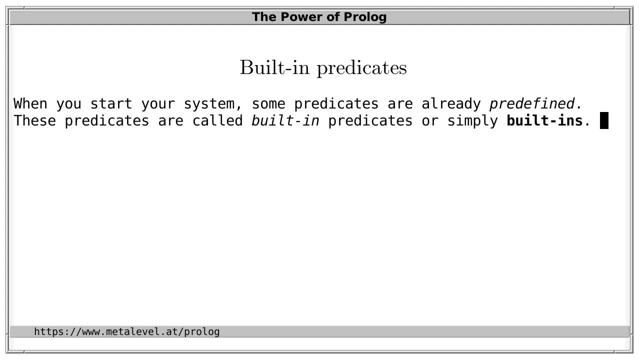 some predicates are already predefined. These predicates are called built-in predicates or simply built-ins. For instance, true is a built-in predicate, It's always true. False is always false. Comma denotes conjunction, So comma of a and b holds if, and only if, a is true. 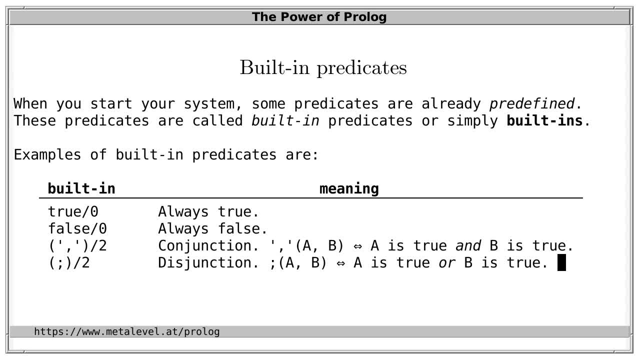 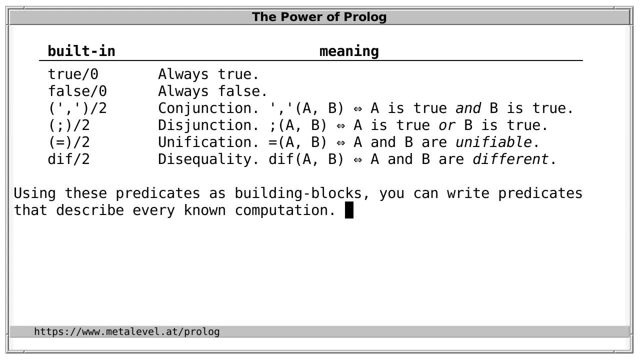 true and b is true. semicolon denotes disjunction, equals denotes unification and div denotes disequality. Using these predicates as building blocks, you can write predicates that describe every known computation And, in fact, if they weren't already available, you could even define most of these built-in. 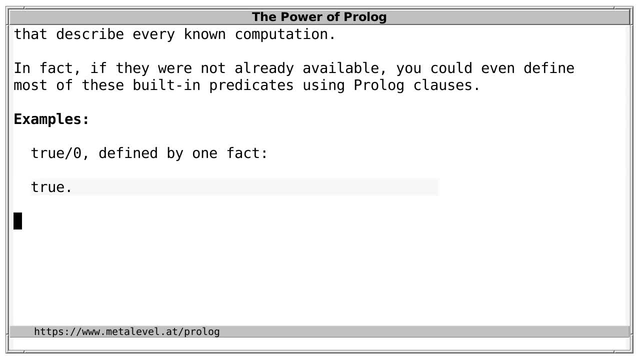 predicates. using Pollock clauses, For instance, we could define the predicate true by simply one fact: true holds. Likewise, we could define equals by one fact. So for all x equals of x and x holds. Of course, since equals is defined as an infix operator, you can also use operator notation. 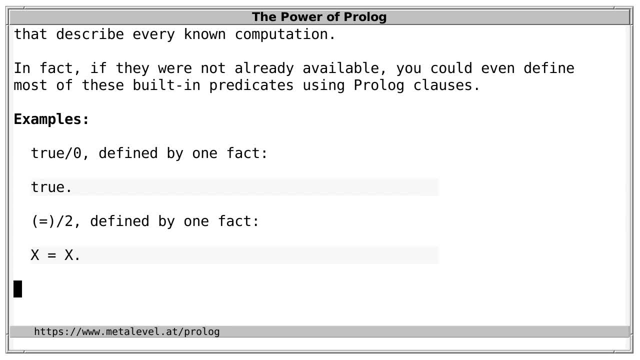 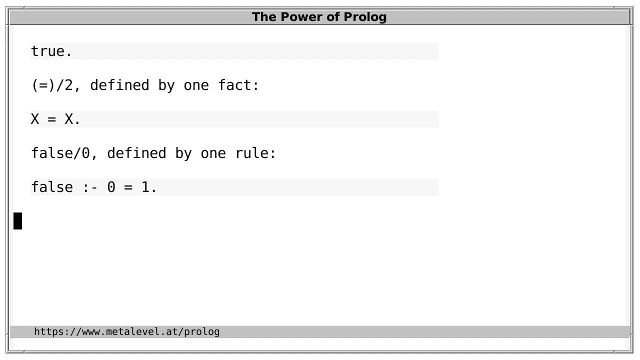 and write this as for all x, x equals, x holds. Okay, False could be defined by one rule. For example, false holds if zero is equal to one, which of course is never the case. So false is always false, And disjunction could be defined by two rules. 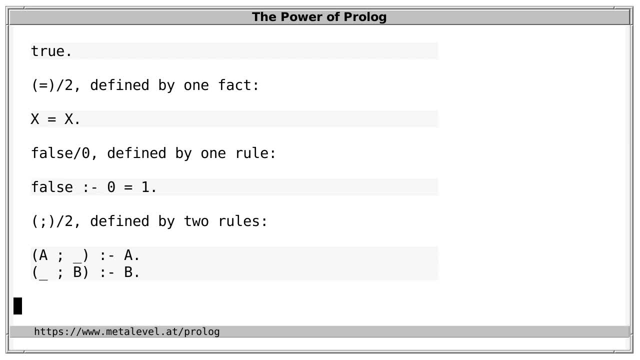 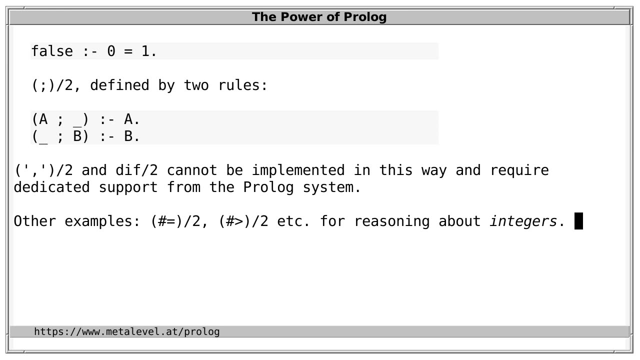 So it holds if a holds or b holds. But some predicates can't be defined in this way. So for instance, comma and div Need special support from the Pollock system. You can't define them yourself. Other examples are predicates. that reason about integers. 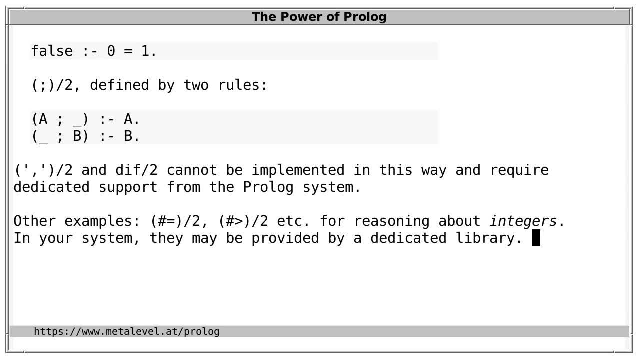 So again, these must be provided by the Pollock system, And in your system they may be provided by a dedicated library, And the Pollock ISO standard specifies what is guaranteed in all systems And of course that's just the minimum that's available in all systems. 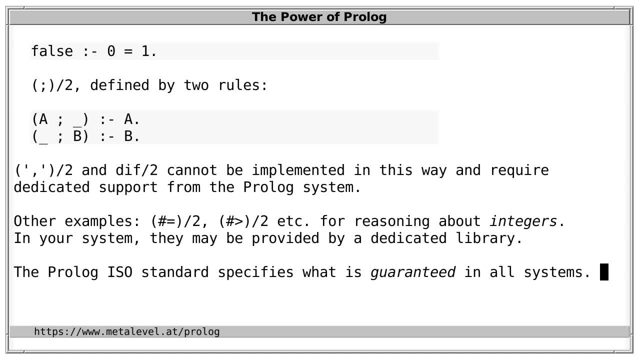 Of course. typically Pollock systems go well beyond the ISO standard and provide many predicates that are not specified in the standard. So they go beyond the bare minimum. For instance, the predicate div was available even in the very first Pollock system. 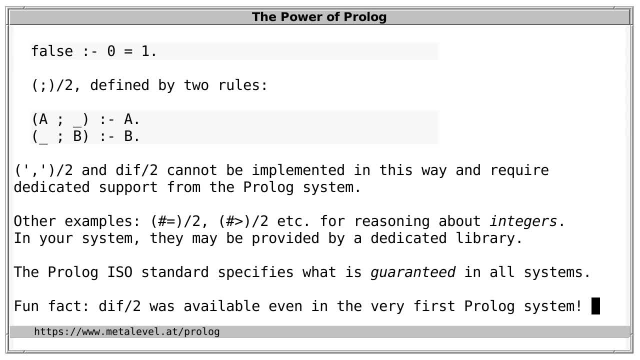 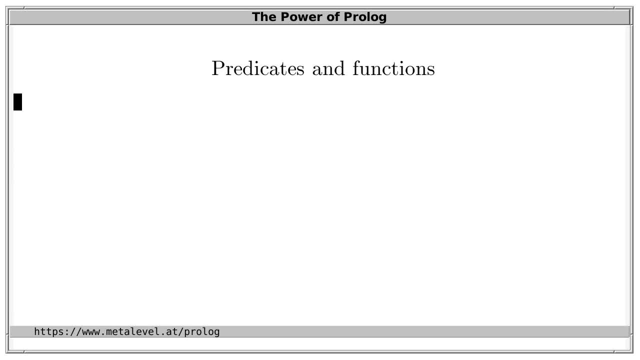 It's not part of the ISO standard, so you can't rely on it being available, But increasingly more implementations do provide it also nowadays. So there is a relation between predicates and functions, Because the predicate p can be regarded as a mapping from domain elements to truth values. 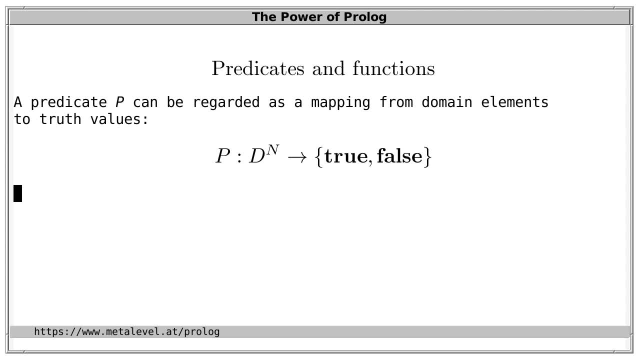 So simply as a function from the n-ary domain to truth, values, true and false, So the predicate holds or not? Conversely, you can also express a function with a predicate. So, for instance, to express the function y is f of x, you could introduce a predicate. 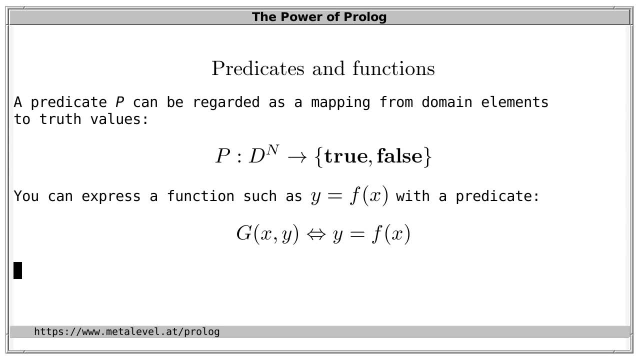 say g of x and y, that holds If, and only if, y is the result of f at x. So predicates can express functions and vice versa. However, predicates are a more natural formalism for defining relations, Because predicates make no distinction between input and output arguments. 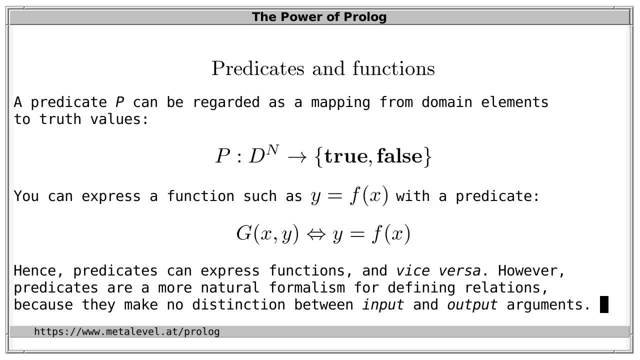 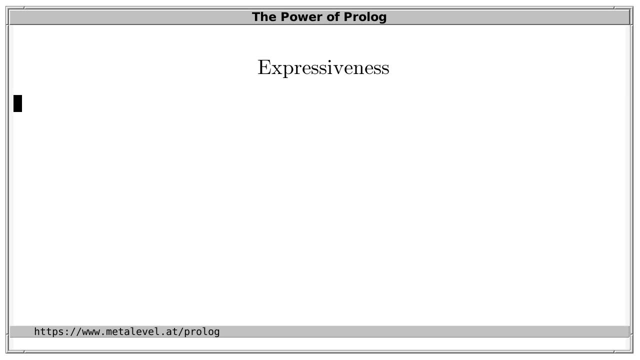 So it's natural to query a predicate in all directions, or in the most general direction, and simply ask the predicate, for which arguments does it hold? So that's it, Whereas a function always implies at least some direction of use. How expressive is this? 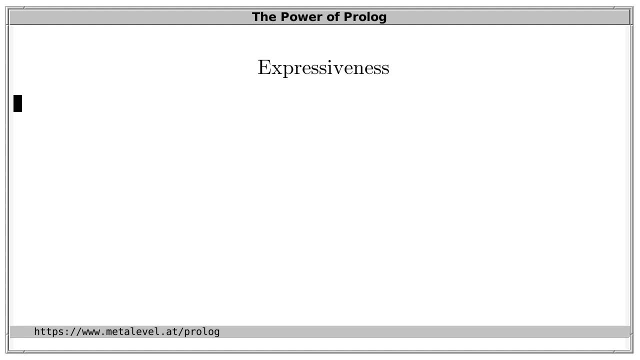 When you start learning Prolog, the language may at first seem very limited to you, Because you have these predicates and you may start by defining some facts and some simple relations. yet it's not clear how to actually express computations in Prolog And 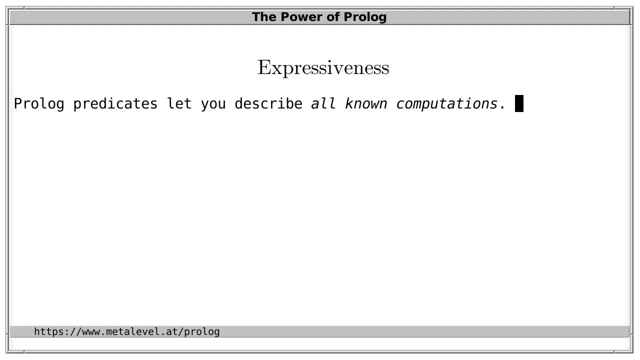 We have already mentioned that Prolog predicates let you describe all known computations. Yet it may not be quite clear how to do this, So I'd like to show you how you can express general computations in Prolog. One way to do this is to simply express the relation between different states of a computer. 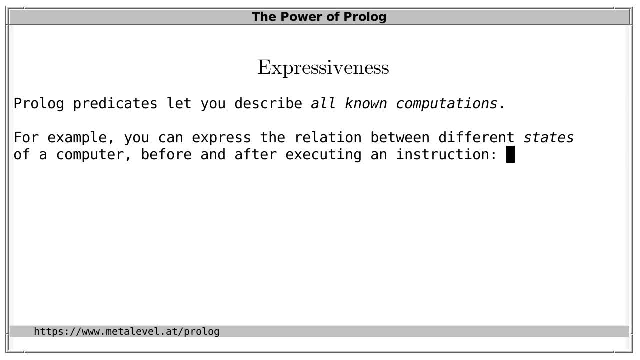 for example, Namely the states before and after executing an instruction. For example, the state before and after executing an instruction. So you could, for example, describe a relation between an instruction- some state is 0, and the next state s- that's obtained by executing the instruction. 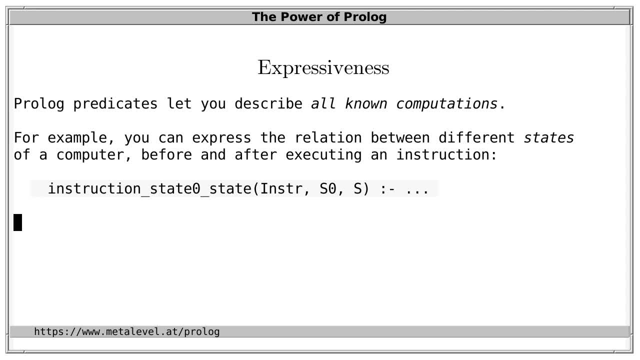 And the instruction can denote everything a computer can do, For instance, write something on the terminal, or write something to a file or at some memory location, And the only thing you have to do to express this Is Is to find a way to represent the state in Prolog, which you can do with a Prolog term. 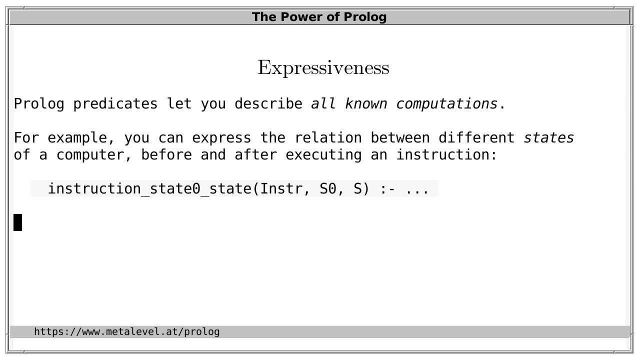 So, for instance, you could have a Prolog term that represents the entire content of the system memory of a computer And then relate this content to the modified content that occurs when the instruction is executed. And once you have such a predicate that relates an instruction to a state,